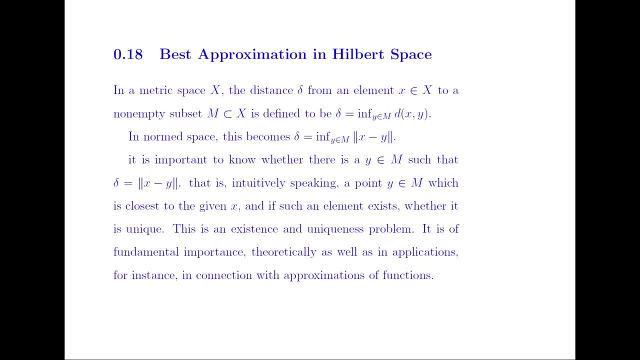 And in norm space this becomes infimum of a norm of x minus y, where y belongs to be M. So it is important to know whether there is y belongs to be a set M such that delta is equal to be norm of x minus y. 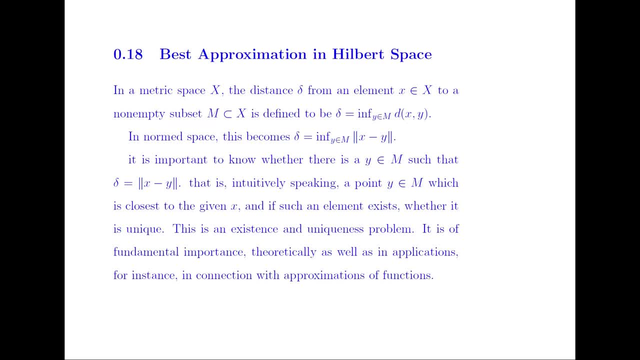 That is, intuitively speaking, a point y belongs to be a set M which is closest to the given point x. If such an element exists, now the question is whether it is unique. So means here we have two problems. are there? 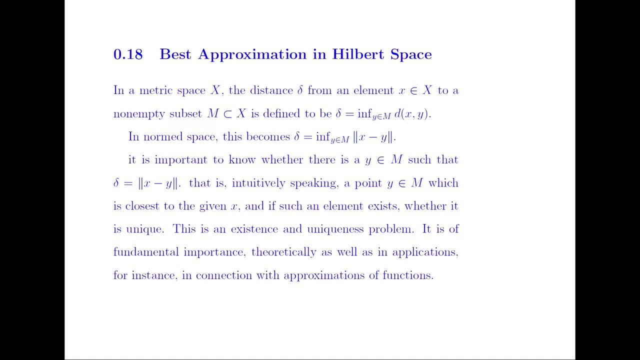 Whether that x is being existing, And if it exists, then the question is whether it is unique or not. So this is an existence and uniqueness problem. It is of a fundamental importance theoretically as well as in applications, for instance in connection with the approximations of functions. 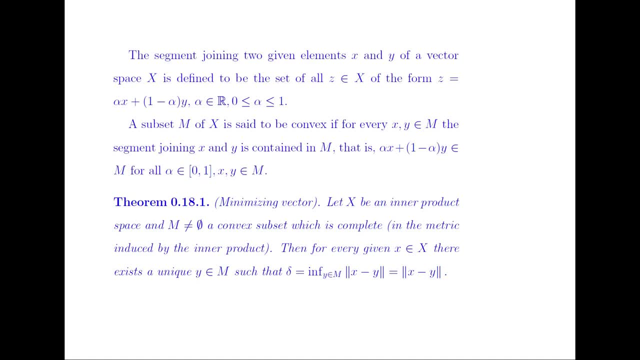 So, before discussing a theorem, we will discuss some definitions. The segment joining the two elements x and y of a vector space, capital, X, is defined to be the set of all z, belongs to be x. of the form, z is equal to be alpha x plus 1 minus alpha y where alpha lies between 0 and 1.. 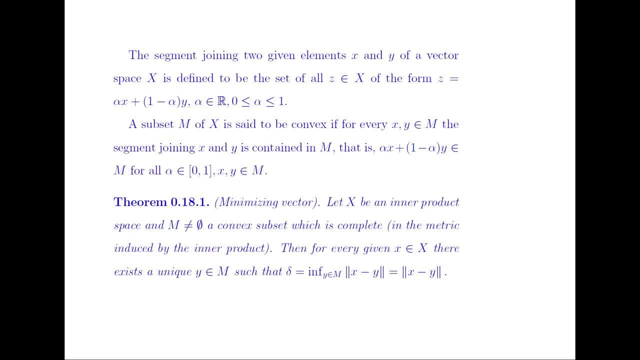 A subset M of a x is said to be convex. if for every x and y belongs to be M, the segment joining x and y is contained in M, That is, alpha x plus 1, minus alpha y belongs to be M. for all alpha belongs to be interval 0, 1, and x and y belongs to be M. 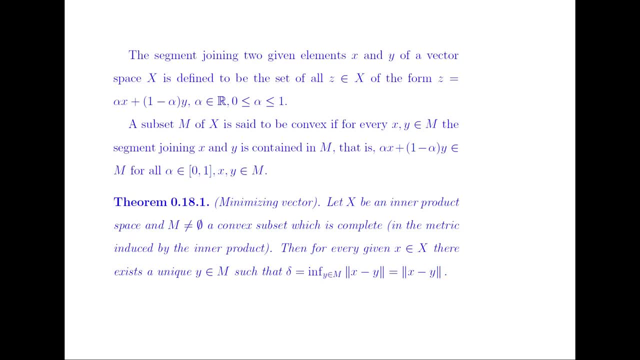 So now we discuss the existence and uniqueness of the minimizing vector in an inner product space. So let x be an inner product space and M is a non-empty convex subset which is complete. Then for every given x belongs to be a set capital X. there exists. a unique y belongs to be a set M, such that delta is equal to be infimum of x minus y, where y belongs to be set M. 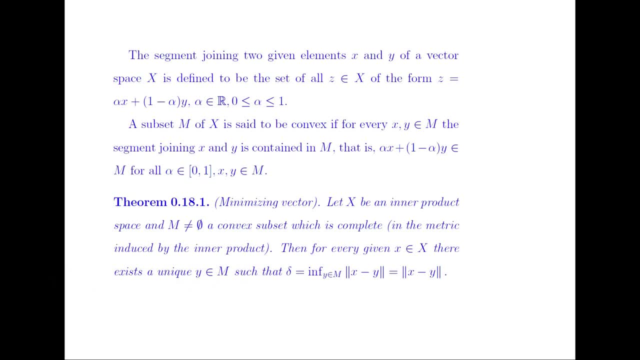 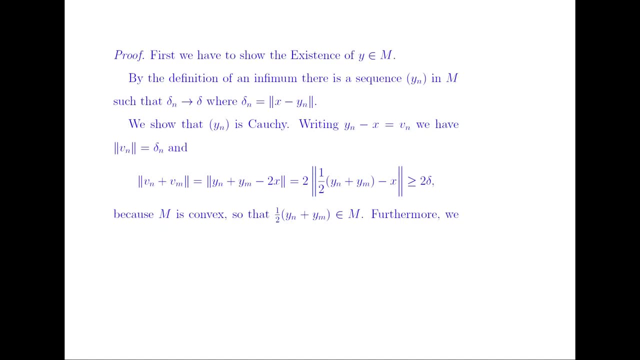 So the proof of this theorem will be divided into two parts. First we will talk about existence, Then we will talk about the uniqueness of this y. First we will talk about the existence of a y. So, by the definition of an infimum, there is a sequence, yn in a capital M, such that delta n converges to be delta. 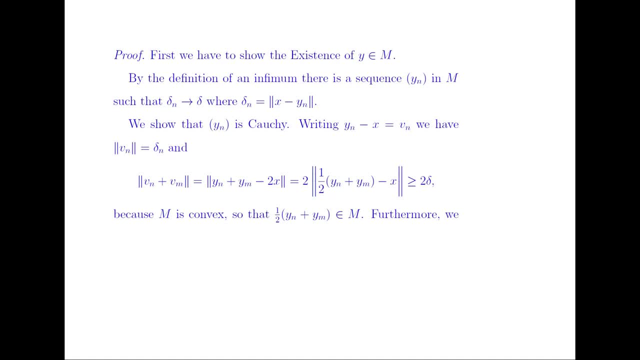 where delta n is equal to be norm of x minus yn. So now we have to show that this sequence is a Cauchy's sequence. Suppose that vn is equal to be yn minus x and we have a norm of a vn is equal to be delta n. 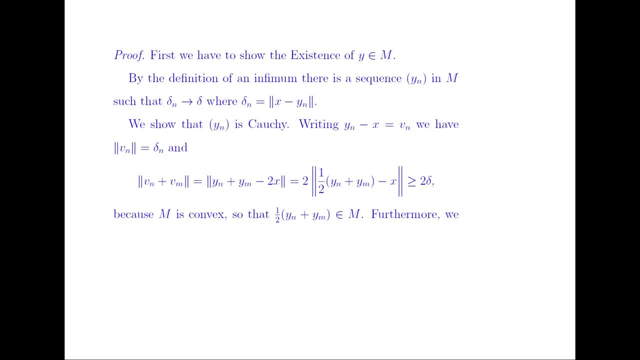 So consider the norm of a vn plus vm, which is equal to be normal norm of a vn plus vm, minus of norm of a to x, while substituting the value of a vn, Taking up a two common out here. so this becomes a norm of half of yn plus ym, minus of x. 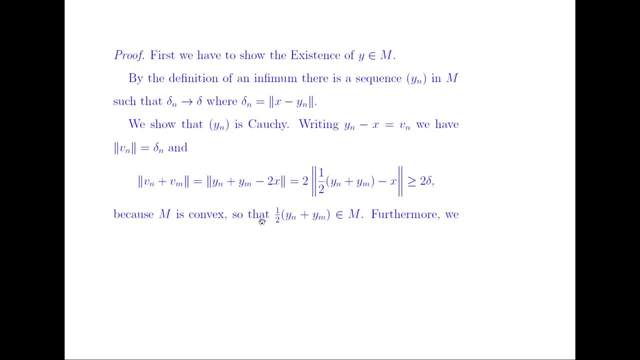 So now here, the set m is a convex and we have a half of a yn plus ym. so y belongs to vm. So this element, this vector, belongs to be a set m. So all those sequences from am minus of ax we have by using a pre-definition, again, this is greater than equal to be delta two times delta. 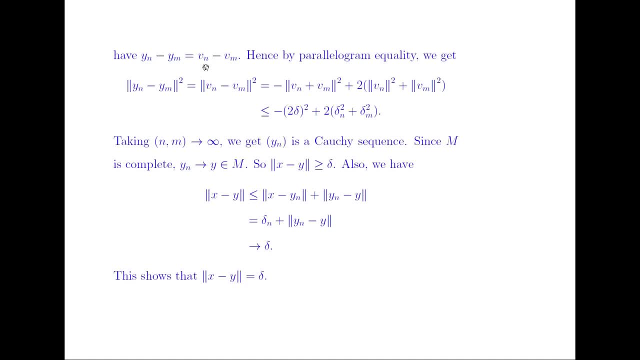 So, furthermore, yn minus ym is equal to be the vn minus the vm and, using up a parallelogram of law, we have considering up a norm of a yn minus ym square is equal to be norm of a vn minus vm square. 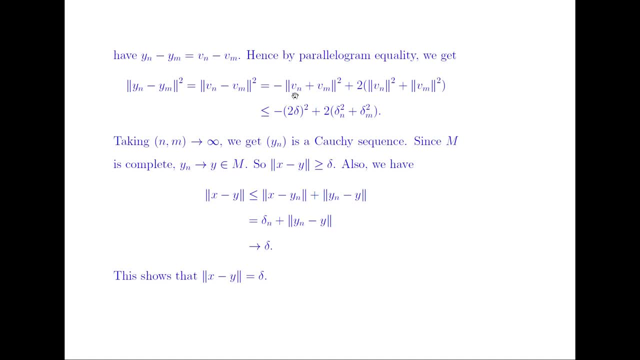 Minus is equal to be minus of norm of a vn plus vm whole square plus two times norm of a vn square plus norm of a vm square. this is by using up a parallelogram of equality. Now this is: vn plus vm is greater than equal to be two times delta, and so minus of this is less than equal to be minus of two times delta square. 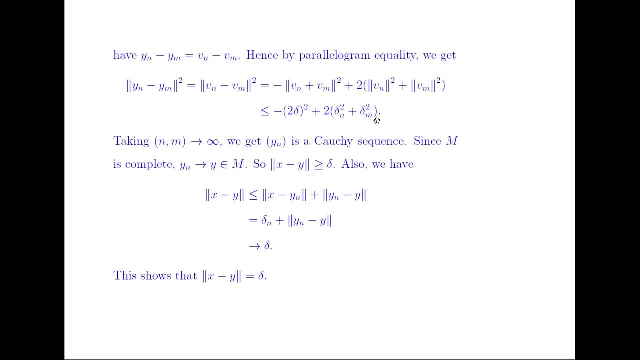 And we have: the norm of a vn square is less than delta n square and norm of a vm square is delta m square. Now, taking up a n and m converges to be infinity. we get this sequence: yn is a cautious sequence And since m is a complete, so this yn converges to be some element of a m, so it converges to be say y. 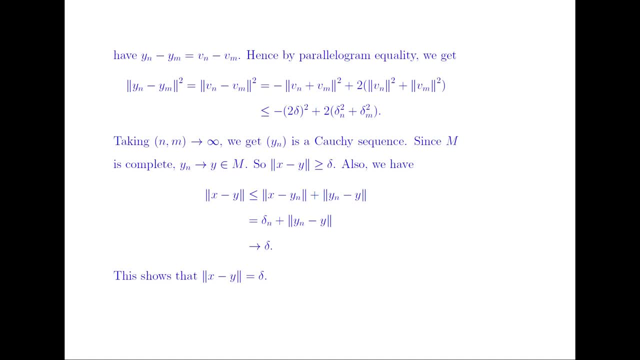 So we have a norm of a x minus y is greater than equal to be delta. So we have the norm of a x minus y is less than equal to be a norm of a x minus yn plus norm of a yn minus y. by using a triangle inequality out here: 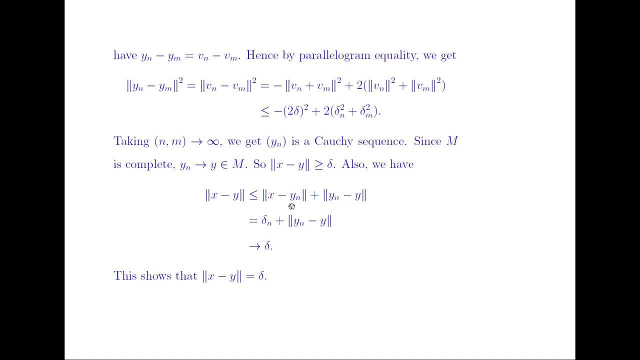 So norm of a x minus yn- we have already talked about this- is equal to be delta n Plus norm of a yn minus y. So this converges to be a delta because the yn converges to be y out here And delta n converges to be delta. 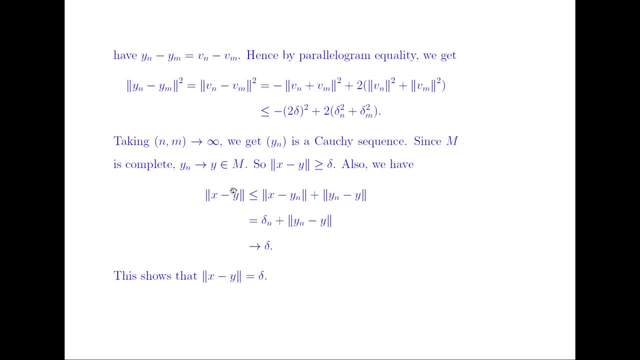 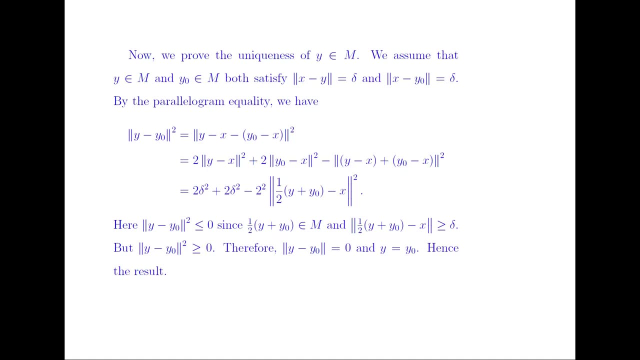 So this shows that this y is being existing up in m. So now we will talk about the uniqueness of such y. So now we prove the uniqueness of y belongs to be m. So assume that there is another element, say y node in m, and satisfying these conditions, norm of a x minus y is equal to be delta and norm of a y. 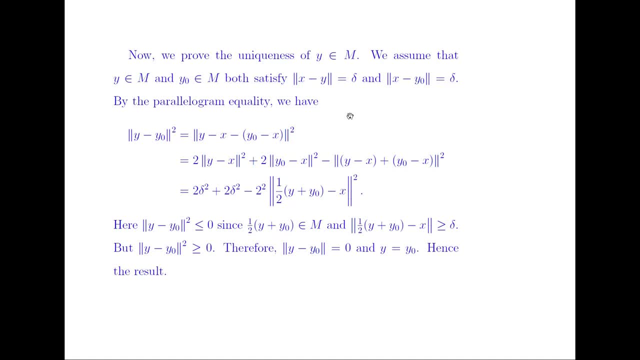 So x minus y node is equal to be delta. So considering up a norm of a y minus y node square which is equal to be norm of a y minus x minus of a y node minus x square, And again using up the parallelogram out here: 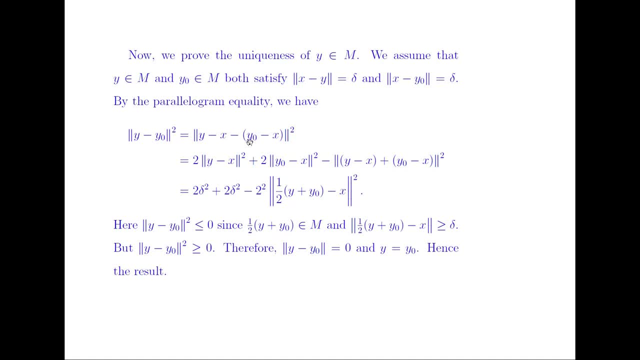 So we can get up: this is a: two times a norm of y minus x square, plus two times a norm of y node minus x square, minus of norm of a y minus x plus y node minus x square, Again using up a. So the properties out here that the half of a y plus y node belongs to be m, because the set m is a convex and this term is greater than equal to be delta. 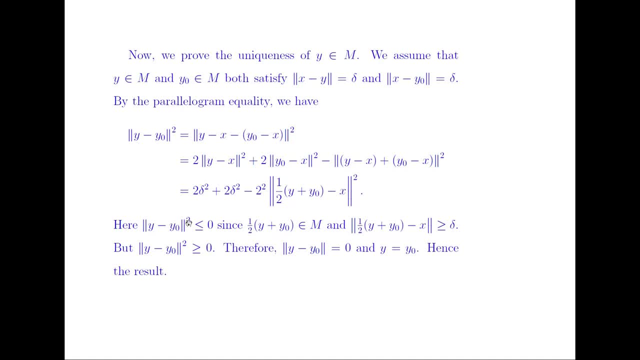 So we found that that the norm of a y minus y node square is less than equal to be zero. But we know the property of a norm is that the norm is always greater than equal to be zero. So we have a norm of a y minus y node is greater than equal to be zero. 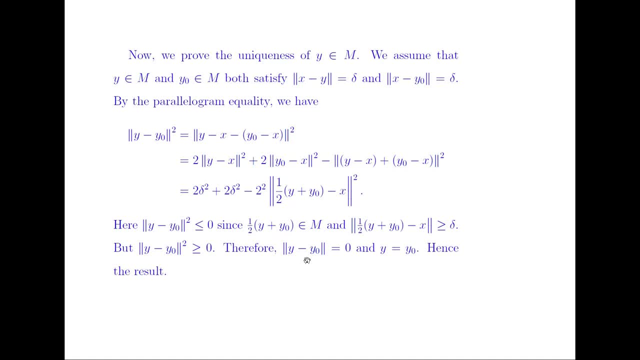 So we have norm of a y minus y node is equal to be zero. That is, the y is equal to be y node. We get the uniqueness of such a y If such y is being existing up, then that y is a unique. 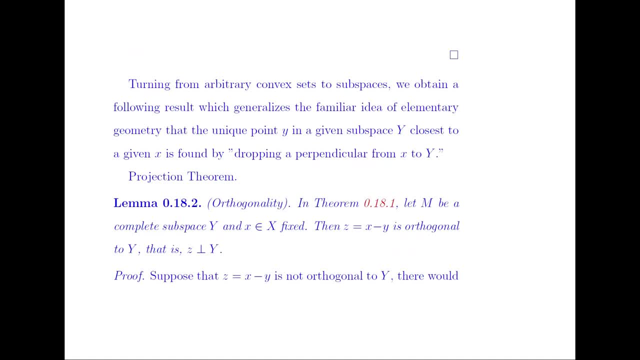 So now, in the previous video we have taken up the convex subsets. So from the convex subsets we are talking about, a subspace is norm. So we obtain a following result, which generalizes the familiar idea of a elementary geometry: that a unique point in a given subspace, y, closes to a. 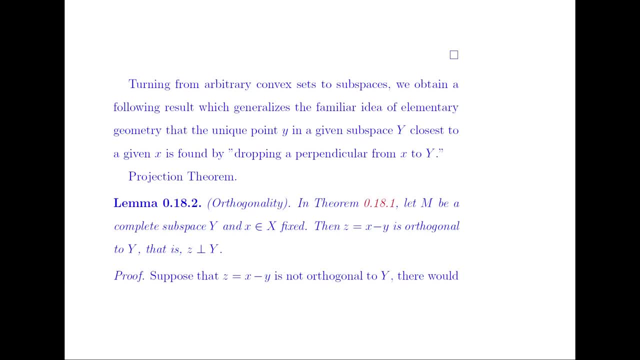 Given x is found by just dropping a perpendicular from x to y, So why it is called a projection theorem. So in the previous theorem, if we consider that the m is a complete subspace of y and keeping the x is being fixed, then the z, which is equal to be x minus y, is orthogonal to y. 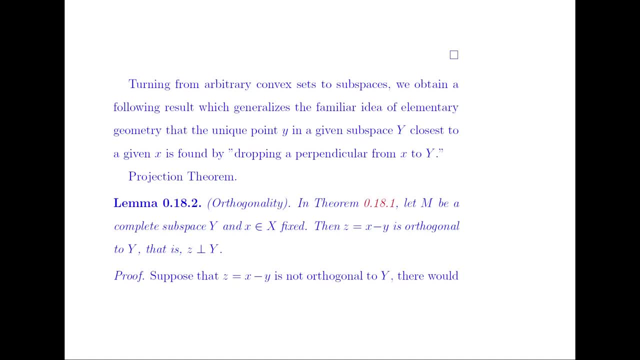 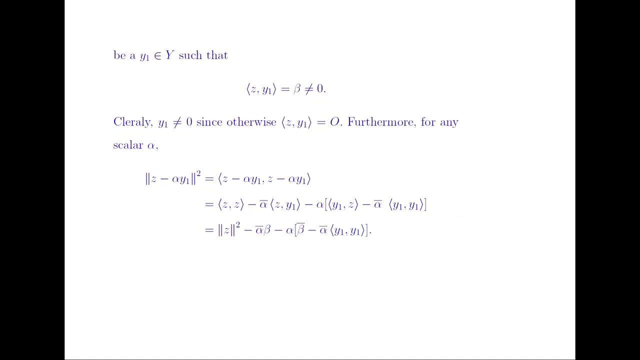 That is, z is perpendicular to y. Now proof of a. So this result will start with a contradiction. suppose that this z is, which is equal to be x minus y, is not orthogonal to y. Now, if it is not orthogonal to the set y, it means that there is just some element y1 in a set y, such that the inner product of a z comma, the y1, is not equal to be zero. 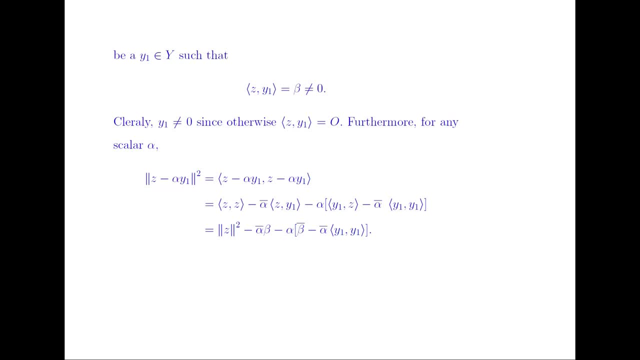 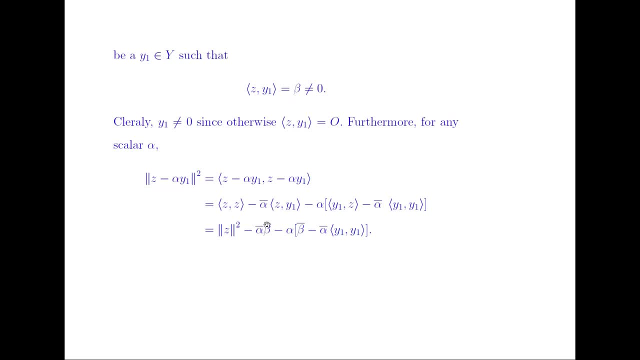 Otherwise the inner product of a z comma y1 is just zero vector. have already considered that this is equal to beta. this is alpha bar into the beta, alpha conjugate into the beta minus of a alpha. now this will become the conjugate of a beta, the beta conjugate minus alpha conjugate into the inner. 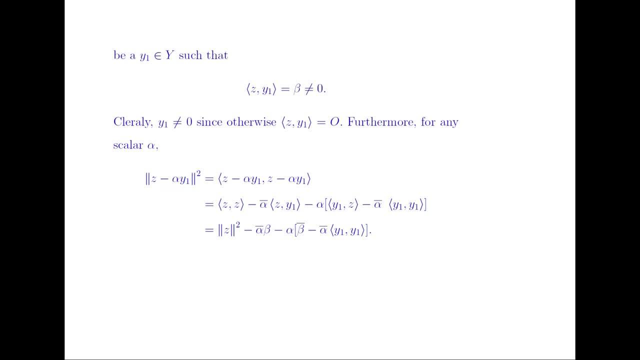 product of a y1 and y1. so, furthermore, we choose this beta bar minus alpha bar into the inner product of a y1. y1 is equal to be 0, then this alpha bar is equal to be the beta bar over the inner product of a y1 comma y1. so we have the 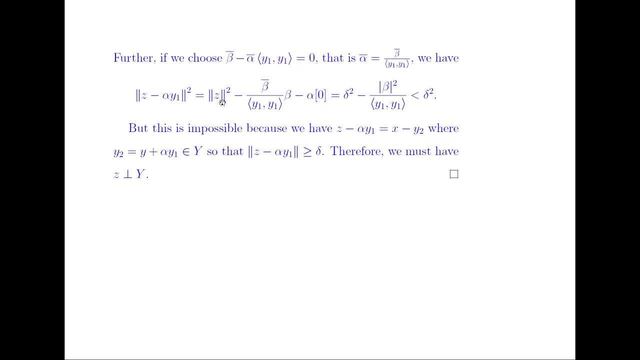 norm of Z minus alpha. y1 square is equal to be norm of Z square minus of substituting the value of alpha bar. here we get this is the beta bar into the beta over the inner product minus alpha into 0, so which is equal to be a delta square minus the norm beta into beta bar is: